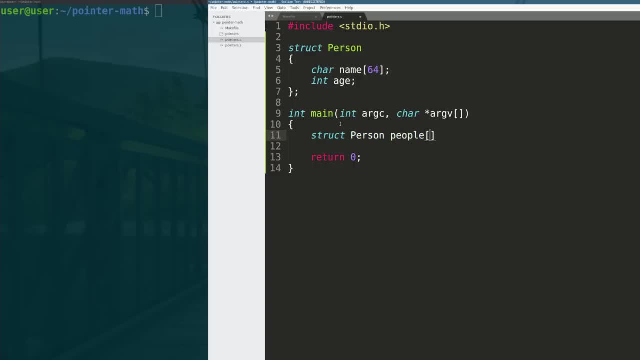 and then you give it a name, So struct person, it's going to be called people. we're gonna have 100 people, So people 100, this will make an array of persons on the stack in our main function. Now, if 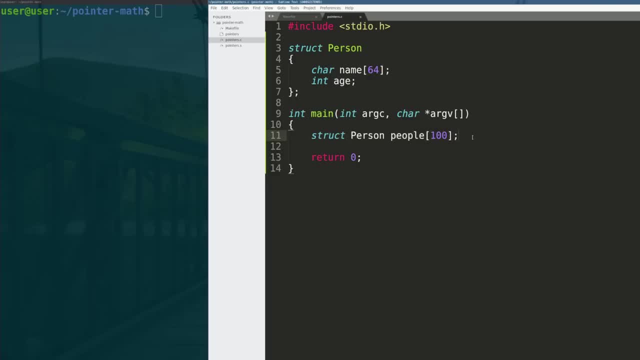 we wanted to edit this. we wanted to go through and either clear the memory of or assign a value to all these people which you act as a cursor as we walk across the array right. So to make a pointer into a structure, we need to say struct, person, which is the type what we're pointing to, and then a star, and then we're. 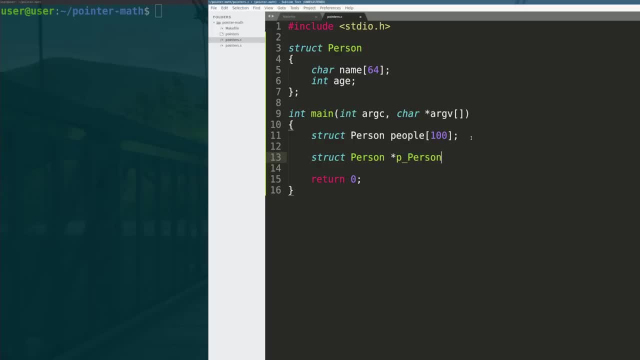 going to say P person, and what does it equal to? It's equal to the address of people. Okay, so what did I say here? this is a person structure pointer, its name is P person and it points to the address of people. 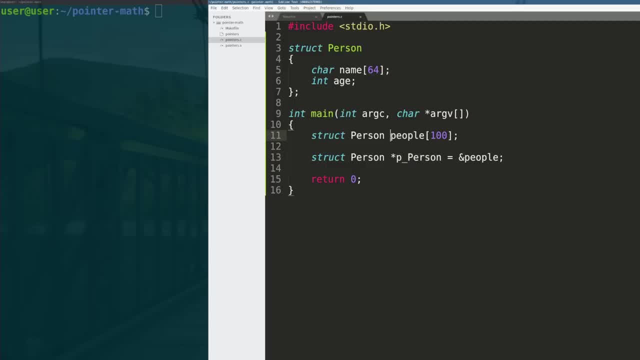 So now, at the end of this line, getting executed p person points to the first person in people. i know we're getting pretty crazy with our english here, but it's gonna, it's gonna make sense. i promise. this points to the base right here. so now, if i wanted to iterate over this list and i wanted to do something to every single person. 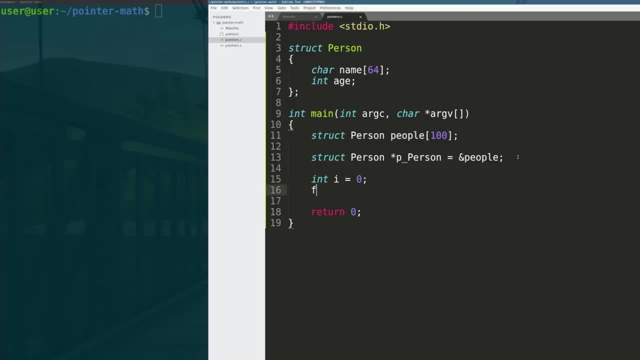 on the list, i would have to do a for loop, right? so int i equals zero, for i equals zero i less than 100, which is the number of people that we have in this list. we're at i plus plus- pretty straightforward. so now here's the problem that people typically get into. so we're going to do our first assignment. 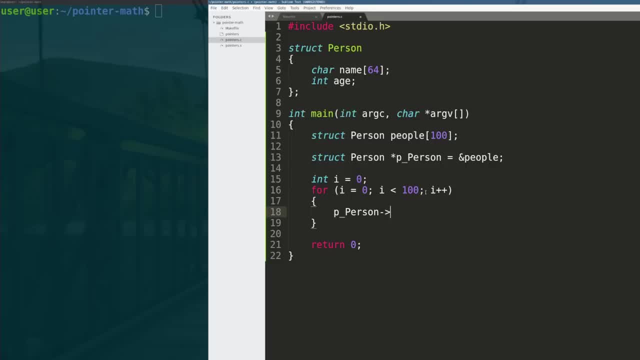 we're going to say that, uh, p person age equals zero. so all i'm doing here is i'm setting their age to zero, i'm clearing the list, and we can do the same thing for name, but we're not going to do that. so the question is: how do we make p person right? our pointer to a person. point to the next. 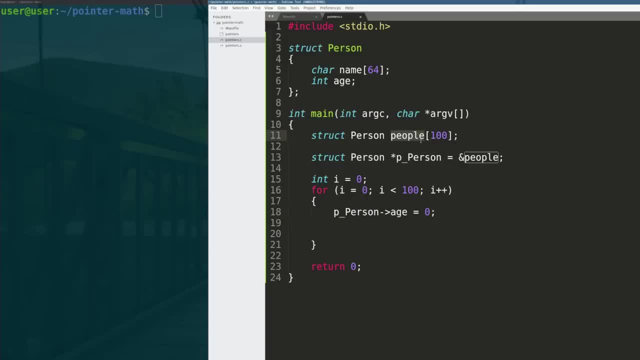 person, right? typically people get very caught up in this and they don't understand the math. they don't understand the math and they don't understand the math. and they don't understand because what? what is a pointer? a pointer is just an integer value that has an address in it, right? 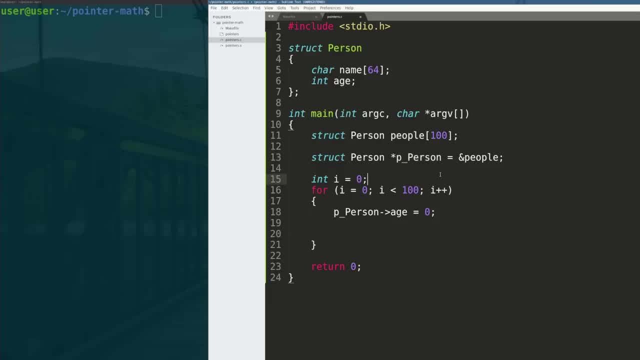 it points to a location. so people would sometimes say, okay, if this is an address, i need to increase it by the size of the element to make the next address the next base. so some people will typically do this: p person plus equals size of struct person, which should be about 68. okay, so this is actually. 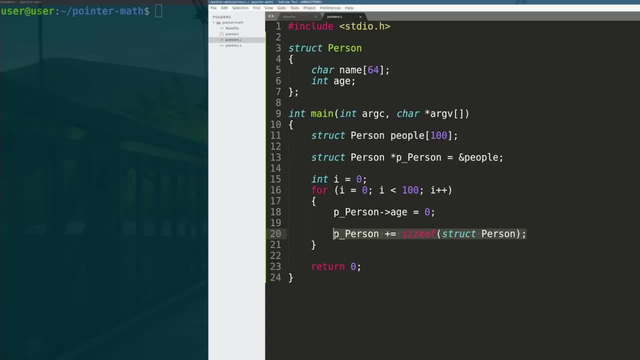 incredibly wrong and will give you crazy bugs. here is why. okay, the c compiler is aware that you are talking about a struct person already, so what it does is it actually multiplies the number that you plus by the size of struct person, so this actually increases it by size of struct person times size. 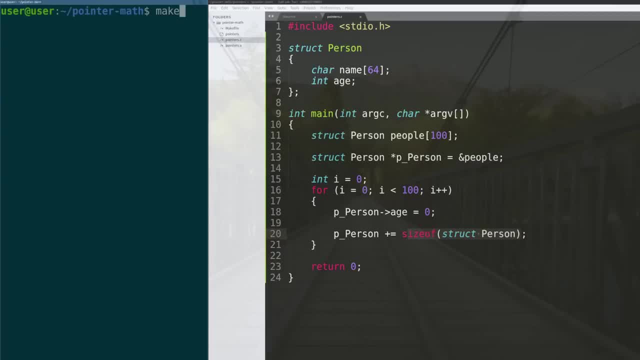 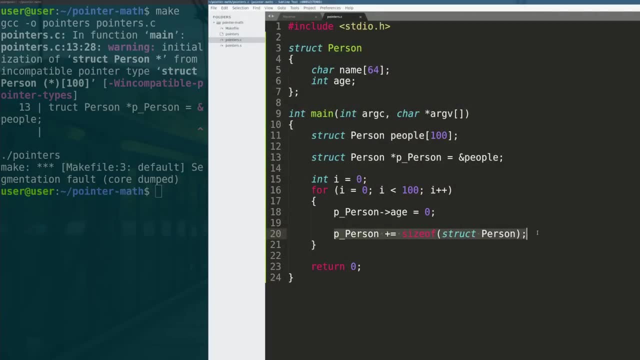 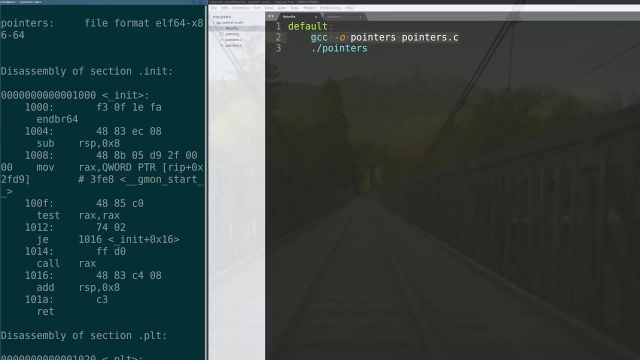 of struct person. so what i actually have going on here is we can use our make file. uh, that's wrong. oh, actually, that's correct. it does crash. so this is going to cause it to crash almost instantly. i have our make file creating our program here, and then i'm actually going to object, dump and pull out the assembly. 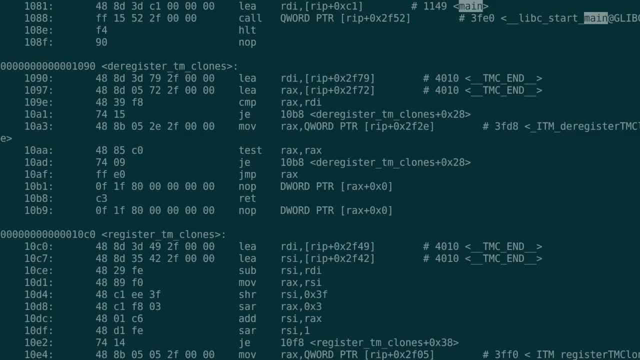 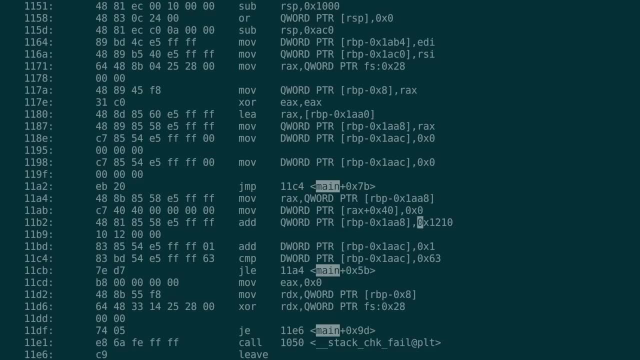 and show you guys what's going on. so we're going to full screen this, we're going to go to our main function, okay, so i know there's a lot going on here, but what you need to see is this part here, right? for some of you guys, this may be a lot of assembly. i know our channel is fairly assembly. 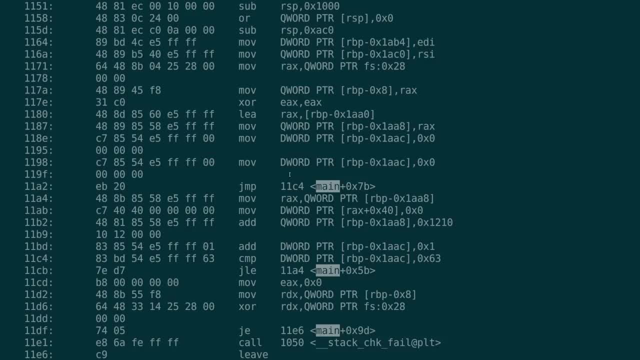 focused. so for those of you that get it, congratulations. if you don't, not a big deal. we're going to walk through here and kind of show you guys what's going on here. we're going to go ahead and show you guys how it's working. so we are in our for loop at this. 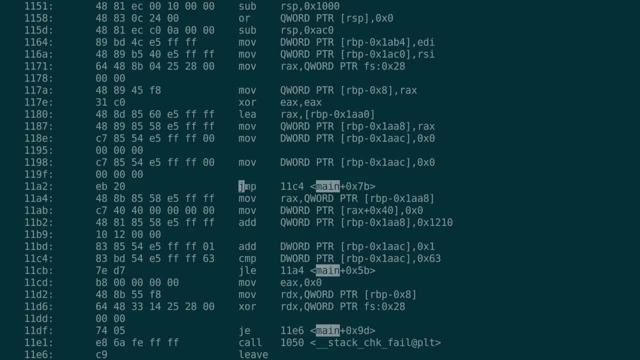 location. this is where we set i equal to zero. we then jump into our for loop at c4. at c4 we compare that i value to hex 63 or 100. if it's less than or equal to it, we go to a4 and then in a4 we add the offset into our array, into rax, and then we set age equal to zero. right. 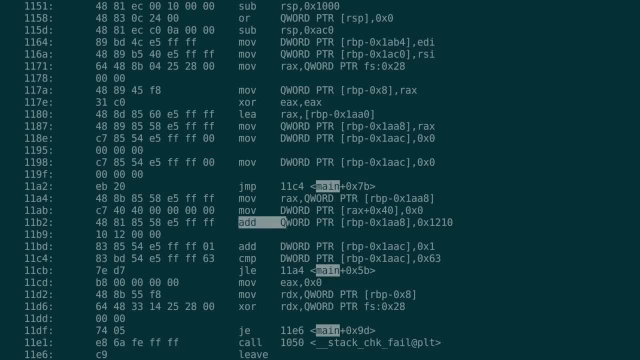 so that's this happening right here. but remember, this at this point is supposed to be after we set the age to zero. we want to increase our pointer by the size of a struct person, but what it's actually doing is increasing it by the size of the struct person multiplied by the size of 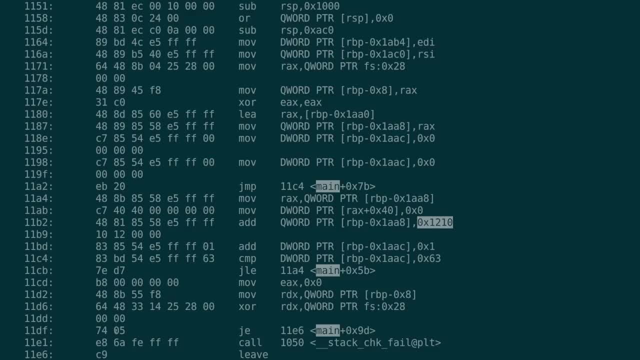 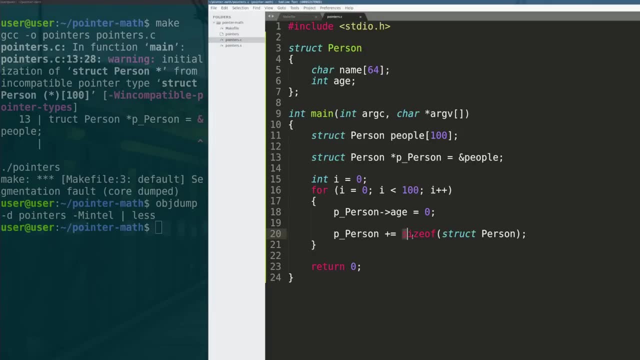 the struct person, because it knows we're already dealing with people. so the actual right answer, the way that we have to index into this array, is simply by doing p: person plus equals one. i know that looks wild. i know that looks like it shouldn't work at all. it's like well. 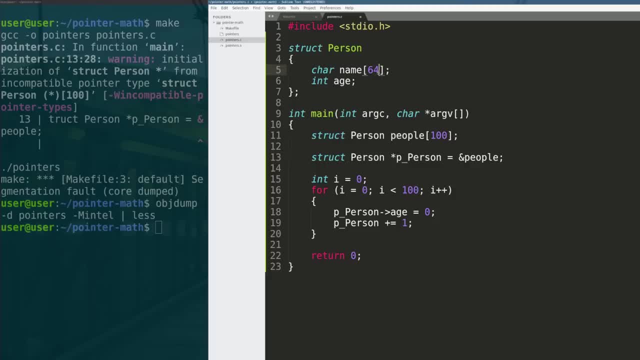 low level learning. isn't that just going to make this point into, like the 63rd character name or whatever? nope, the c compiler is actually doing you an absolutely huge favor and it knows. hey, man, we're cool. i know you're dealing with people. i know that when you say plus one, you want to go. 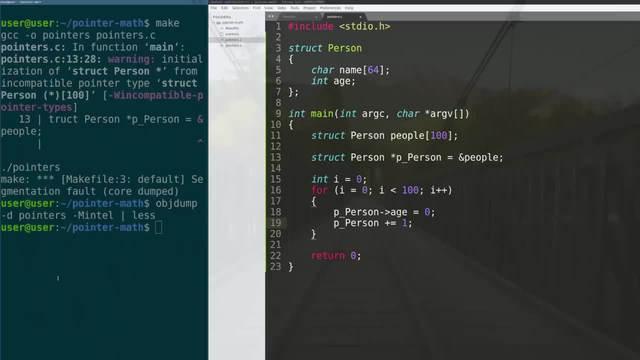 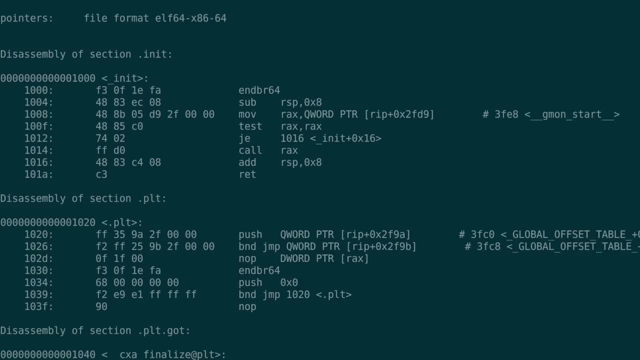 to the next one and not, you know, the next byte in the array, so we can actually make that real quick note that it doesn't crash this time. and then we're actually going to go in and we're going to object, dump that value and we're going to go to main. we're going to find our loop here. so here's. 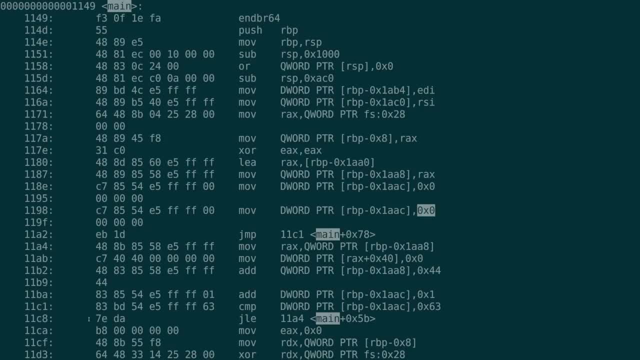 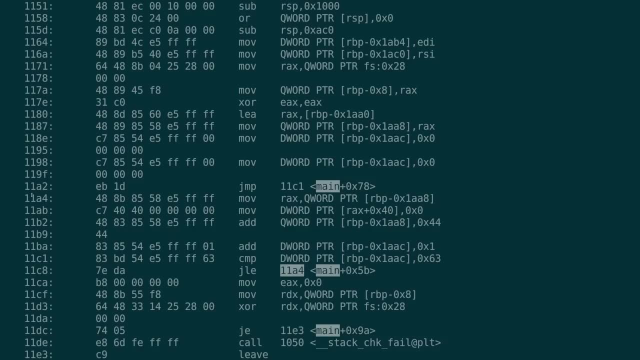 us setting i equal to zero. we're going to jump down to ac. excuse me, now we're going down to c1, c1 here compared to 63. if not, go to a4, a4, boom, boom. okay. now we're going to add hex 44. guys, what is hex 44? 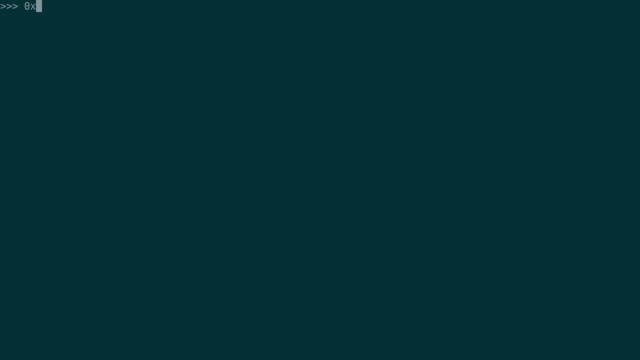 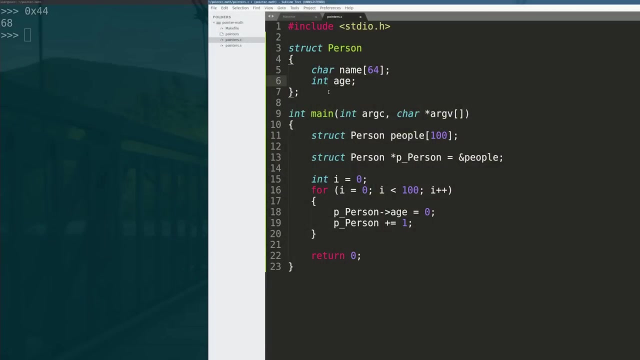 let's ask python 68. wow, did i not say that 68 was the exact size of struct person? it all comes together. so what we can do here now is keep going with our list and we can do things like p, person, uh, name of zero equals zero. that will null, terminate the value, so that we don't get any. 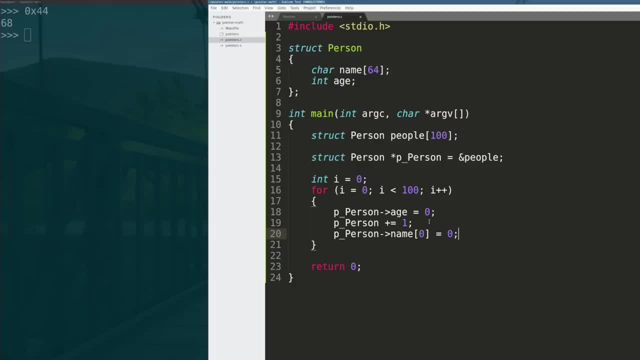 output from it. we can do a whole bunch of cool stuff like that. so, guys, i hope that this video did a little bit for you. it showed you kind of why pointer arithmetic comes off as so complicated, but at the end of the day it's really not that hard. it's just the compiler is already aware of. 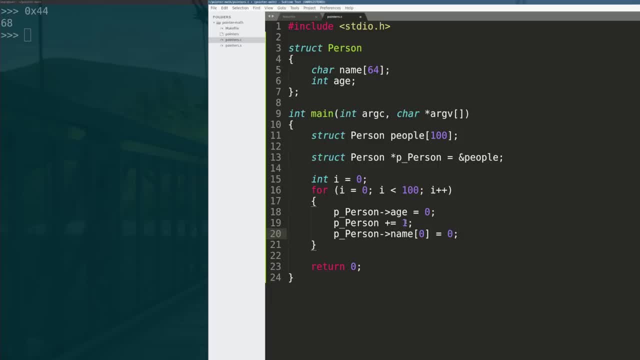 what you're talking about. let it do the work for you. we can jump to the next one and we're going to jump over every other person. we can go to every third person or every fourth person, because the compiler is already aware of what you're talking about when you're doing pointer arithmetic guys. 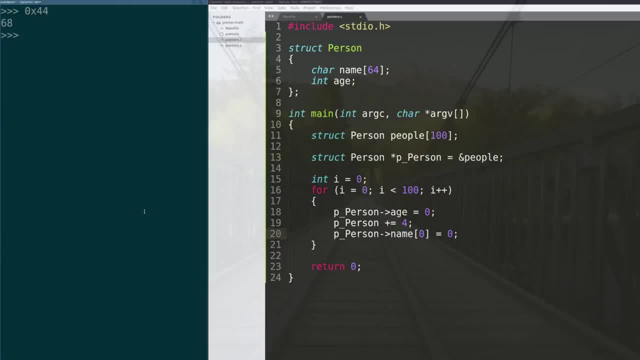 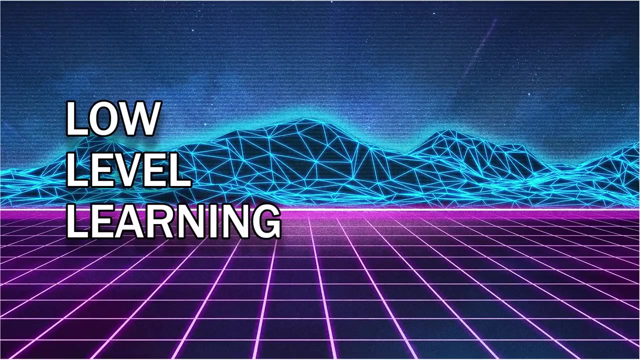 if you like this video, if you learned something, or if i made your life a little bit easier, do me a favor, hit like, hit, subscribe and i'll see y'all in the next video. still crashed, not sure why. take care you.